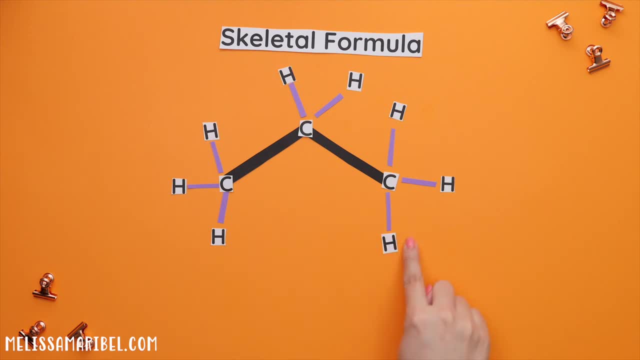 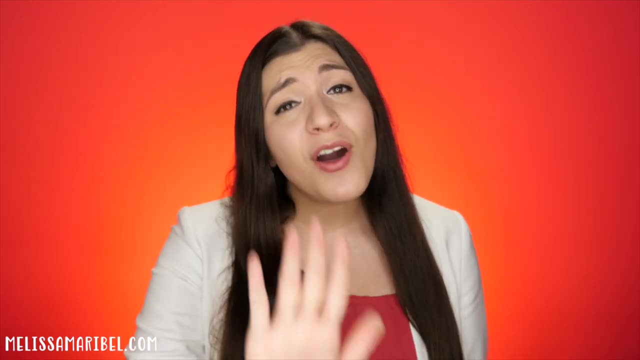 And this last carbon already has one bond, so we need three more bonds, so three more hydrogens. To make sure you get this down and don't miss anything on your exam, make sure to pause the video and try this question out, and we'll go over the answers together. 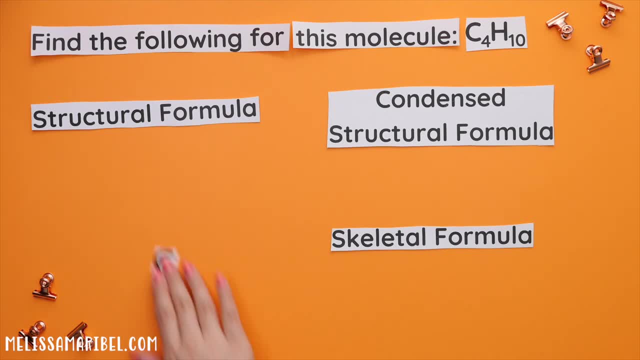 Okay, here are the answers. The structural formula consists of four carbons and ten hydrogens, So this first carbon needs three hydrogens. Next carbon has two bonds, so it needs two hydrogens. Same goes for this carbon And this last carbon has one bond, so it needs three hydrogens. 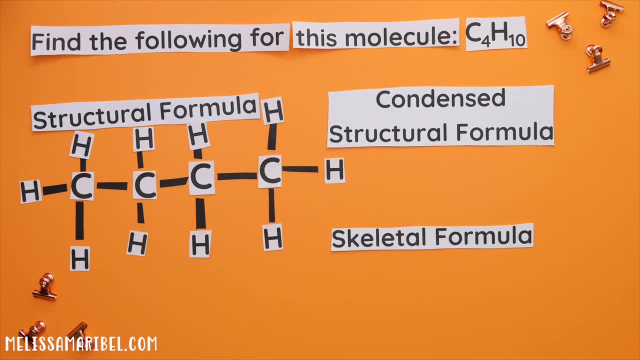 So this is our structural formula. Using the structural formula we'll write the condensed structural formula where this first carbon has one bond, so it needs three hydrogens. Where this first carbon has three hydrogens, so CH3.. The next carbon has two hydrogens, so CH2.. 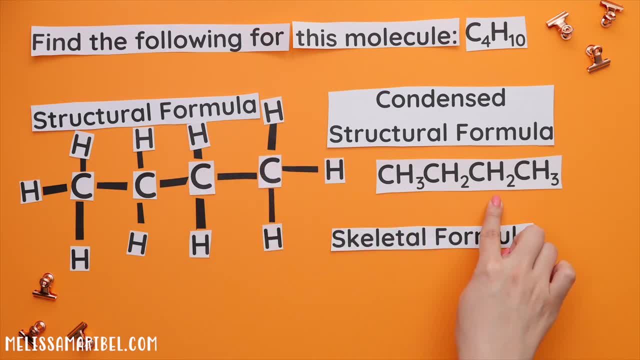 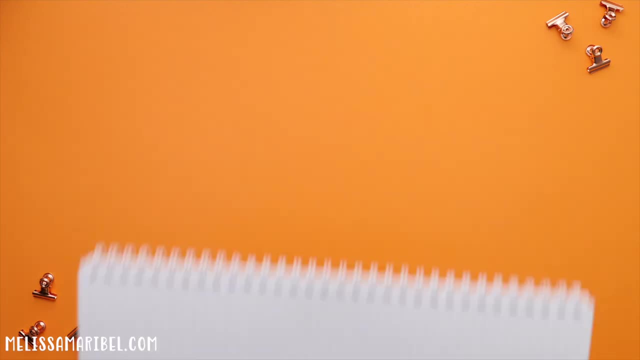 Same for the next carbon, so CH2.. And the last carbon has three hydrogens, so CH3.. This is our condensed structural formula. Now for the skeletal formula. Since there are four carbons, we need four points. There is a trick to drawing this right each time. 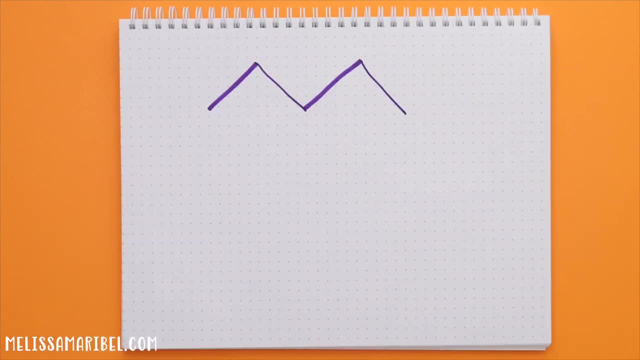 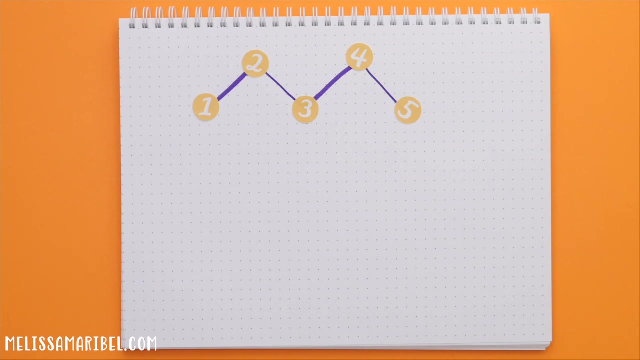 If you were to count one, two, three, four. we actually drew too many carbons. We drew one, two, three, four, five, but we just wanted four. So if you count to one, less carbon than what you're originally looking for. 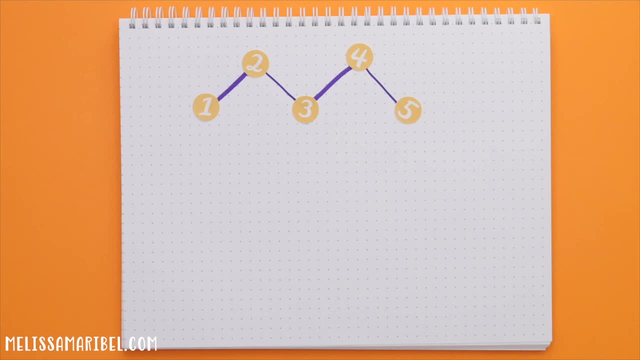 then you will draw the correct amount of carbons each time. So in our case we will count to three when drawing the lines. So one, two, three, And we really have one, two, three, four. This is the correct skeletal formula. 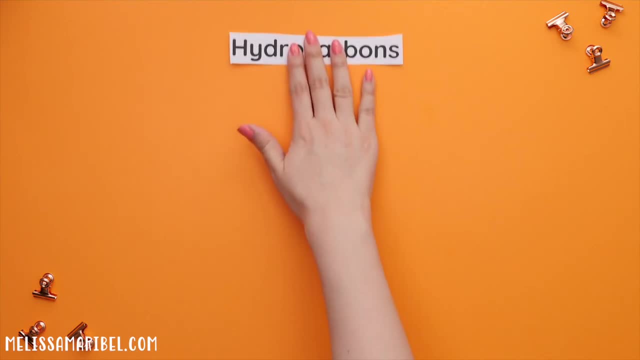 These molecules that we are working with are called hydrocarbons. A hydrocarbon consists of only hydrogens and carbons. There are different types of hydrocarbons. This is based on the type of bonds that are between the carbon atoms. Alkanes have single bonds.